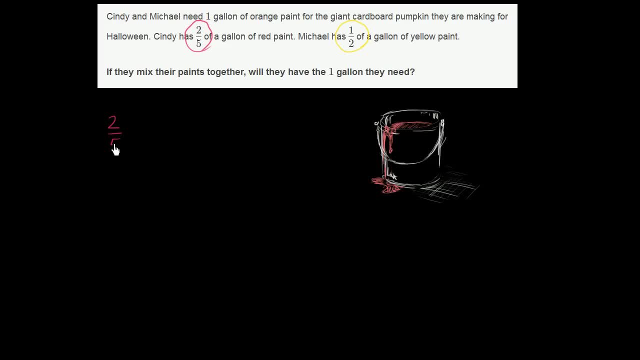 So let's think about that. We're going to add the 2 fifths of a gallon of red paint and we're going to add that to half a gallon of yellow paint And we want to see if this gets to being one whole gallon. 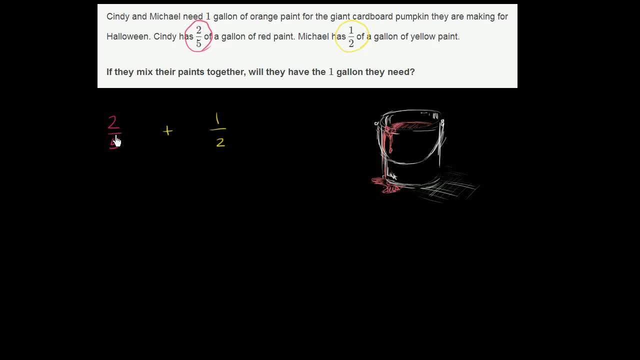 So whenever we add fractions right over here, we're not adding the same thing. Here we're adding 2 fifths, Here we're adding 1 halves. So in order to be able to add these two things, we need to get to a common denominator. 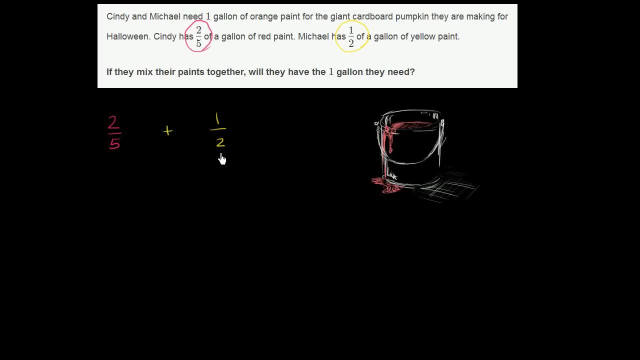 And the common denominator, or the best common denominator to use, is the number, that is, the smallest multiple of both 5 and 2.. And since 5 and 2 are both common, both prime numbers, the smallest number is just going to be their product. 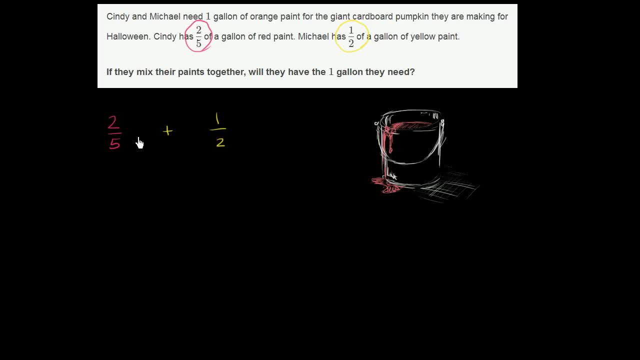 10 is the smallest number that we can think of. that is divisible by both 5 and 2.. So let's rewrite each of these fractions with 10 as a denominator. So 2 fifths is going to be something over 10.. 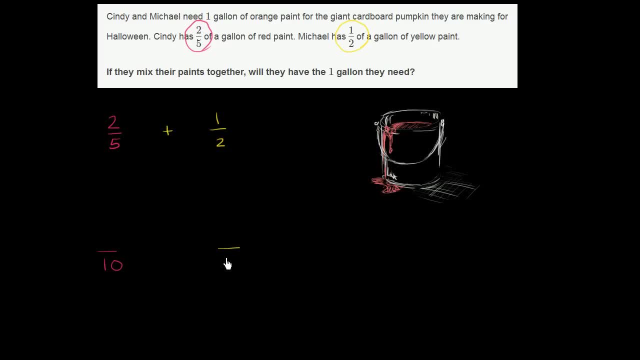 And 1 half is going to be something over 10.. And to help us visualize this, let me draw a grid with tenths in it. So that's that, And that's that right over here. So each of these are in tenths. 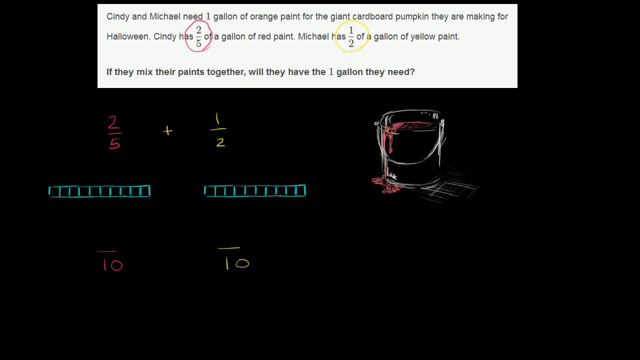 These are 10 equal segments this bar is divided into. So let's try to visualize what 2 fifths looks like on this bar. Well, right now it's divided into tenths. If we were to divide this bar into fifths, 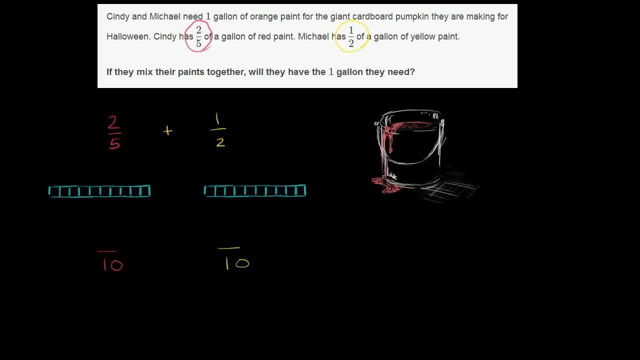 then we're going to have 1 division, 2, 3, 4.. So notice, if you go between the red marks, you are going. these are each a fifth of the bar if you go between the red marks. 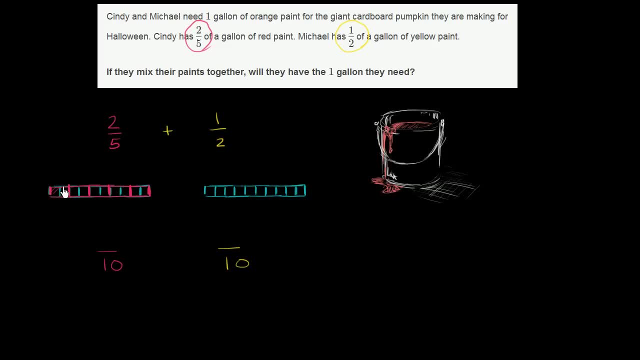 And we have two of them, So we're going to go 1 and 2.. This right over here, this part of the bar, represents 2 fifths of it. Now let's do the same thing for 1 half. So let's divide this bar exactly in half. 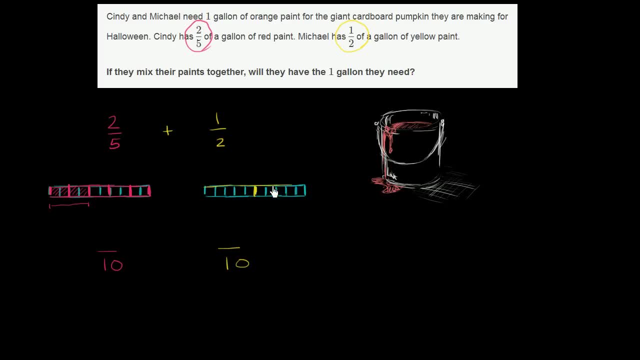 So exactly in half. So let me do that. So I'm going to divide it exactly, Exactly in half, And 1 half literally represents 1 of the 2 equal sections. So this is 1, 1 half. Now to go from fifths to tenths. 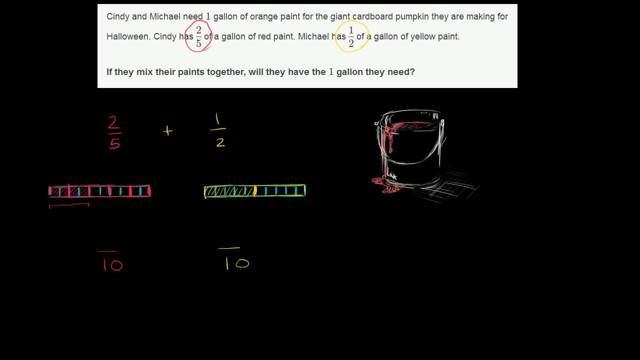 you're essentially taking each of the equal sections and you are multiplying by 2.. So, to go from fifths to tenths, you're multiplying by 2.. You have 5 equal sections. You split each of those into 2. So you have twice as many. 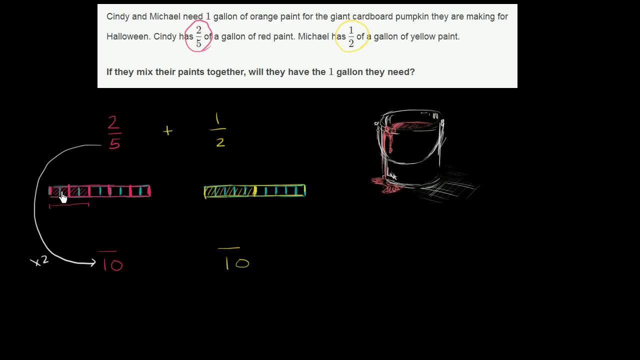 And you now have 10 equal sections. So those 2 sections that were shaded in. well, you're going to multiply by 2. the same way, Those 2 are going to turn into 4 tenths, And you see it right over here. when we shaded it initially, 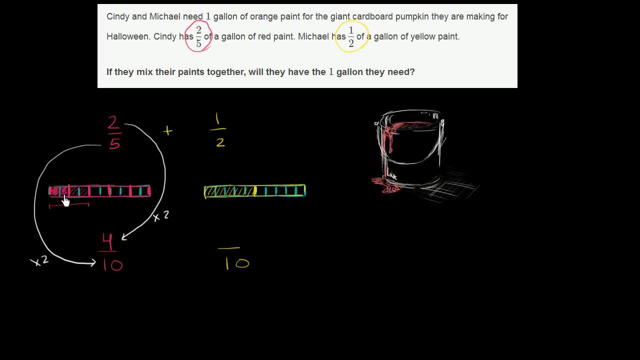 If you look at the tenths, you have 1 tenth, 2 tenths, 3 tenths and 4 tenths. Let's do the same logic over here. If you have 2 halves and you want to make them into 10. 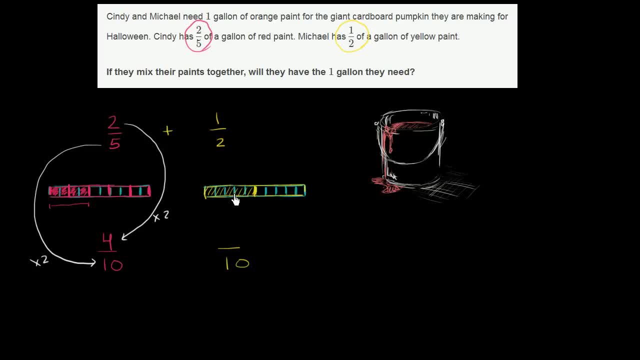 tenths. you have to take each of the halves and split them into 5 sections. You're going to have 5 times as many sections. So to go from 2 to 10, we multiply by 5.. So similarly that 1 shaded in section in yellow. 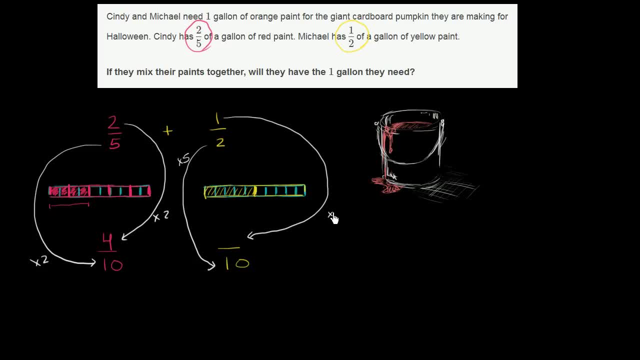 that 1 half is going to turn into 5 tenths, So we're going to multiply by 5.. Another way to think about it: whatever we did to the numerator, or whatever we did to the denominator, we have to do to the numerator. 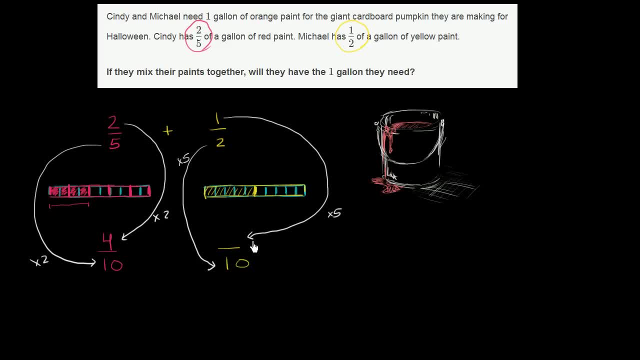 Whatever we did to the denominator, we have to do to the numerator, Otherwise we're changing the value of the fraction. OK, So 1 times 5 is going to get you to 5. And you see that over here when we shaded it in. 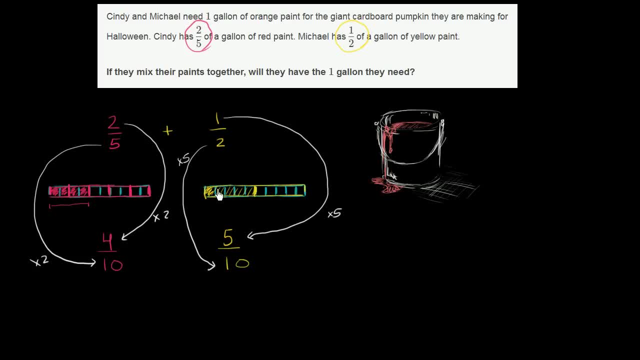 That 1 half, if you look at the tenths, is equal to 1,, 2,, 3,, 4, 5 tenths. And now we are ready to add these two things: 4 tenths plus 5 tenths. 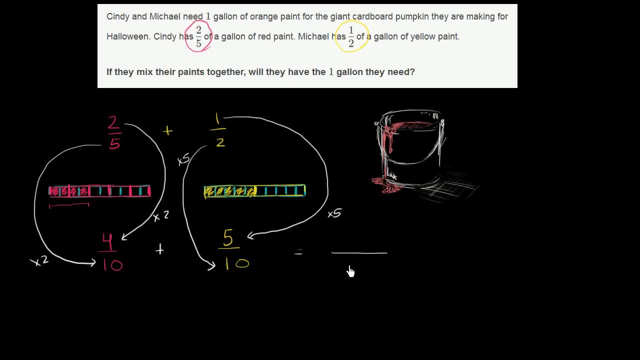 Well, this is going to be equal to a certain number of tenths. It's going to be equal to 4 plus 5 tenths, 4 plus 5.. 4 plus 5 tenths, And we can once again visualize that.